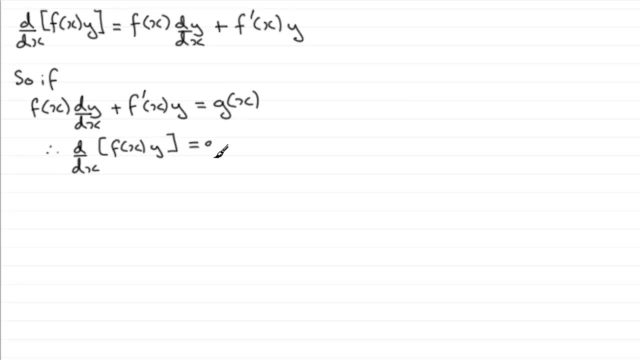 And that would equal Our function g of x. Now, if I integrate both sides with respect to x, then this side is just going to go to f of x times y, and the right-hand side would be just simply the integral of g of x with respect to x. 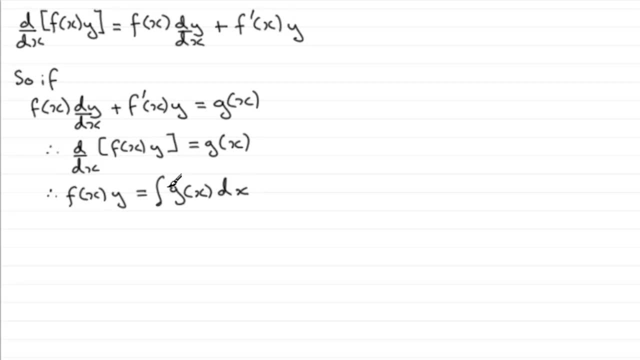 So if we have something like this, and assuming that we can integrate this very easily, then we can get a solution. We can get a solution to our differential equation. And just to give you an example of how this works, let's just take this one here. 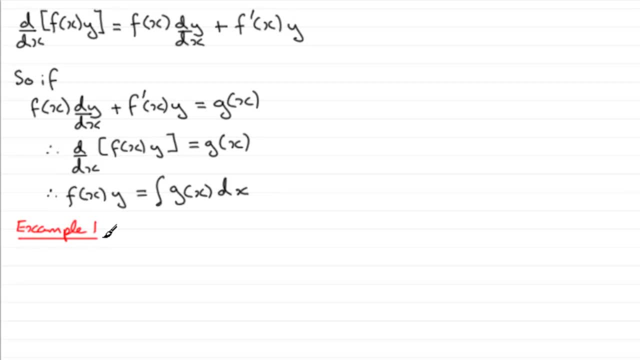 We'll just say example one. So we need to have something that's got this format. So if I had say x to the power 4, dy by dx, and this was say my f of x, then the next term must be f dash of x. 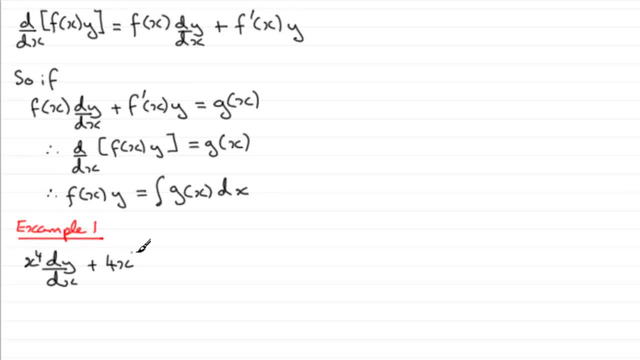 So in other words, 4x cubed multiplied by y And this can equal, say, any function of x, g, of x. I've got here. Let's say it equals e to the power 2x, Then I should be able to solve this by this technique here. 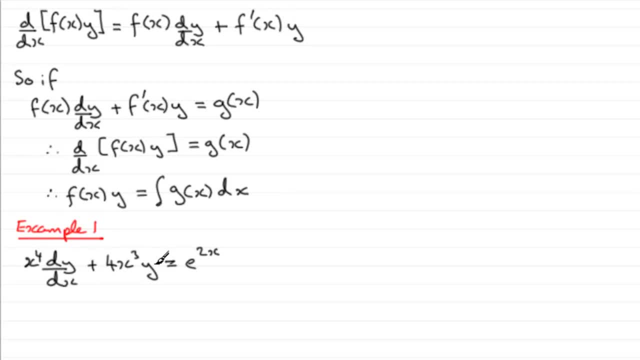 Because on the right-hand side of this equation, this is exactly the same as saying that it's the differential with respect to x of x to the power 4, my f of x multiplied by y. Because if you differentiated this by the product rule, 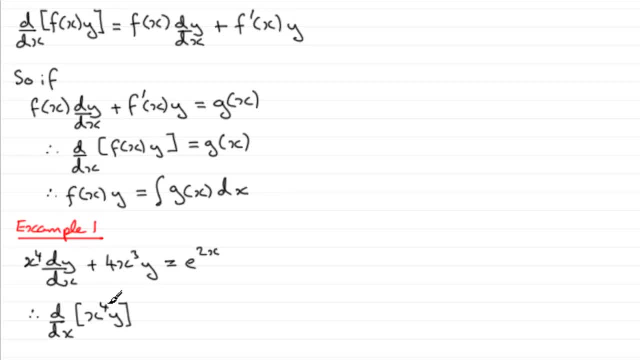 you would get this result: First part x to the power 4, times the differential y with respect to x, that would be x to the 4, dy dx, And then plus the differential of this part, which would be 4x cubed, and then you multiply it by the y. 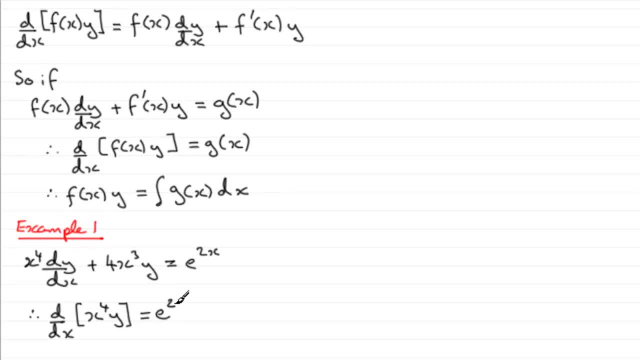 And that would now equal, in this example, e to the power 2x. Now, if we integrate both sides with respect to x, then what we're going to have here on the left is just simply x to the power 4 multiplied by y. 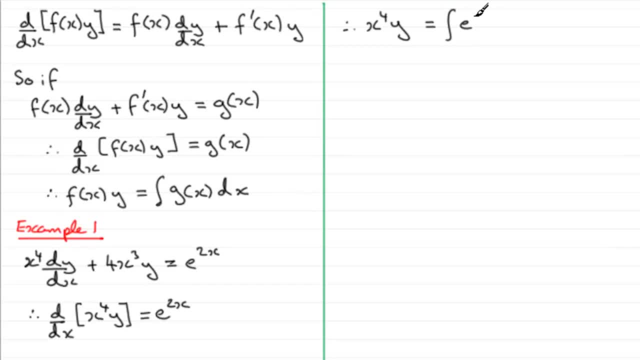 And that's going to equal the integral of e to the power 2x, integrated with respect to x. And so therefore, what we have is x to the power 4 times y equals, and the integral of e to the power 2x is a half e to the power 2x. 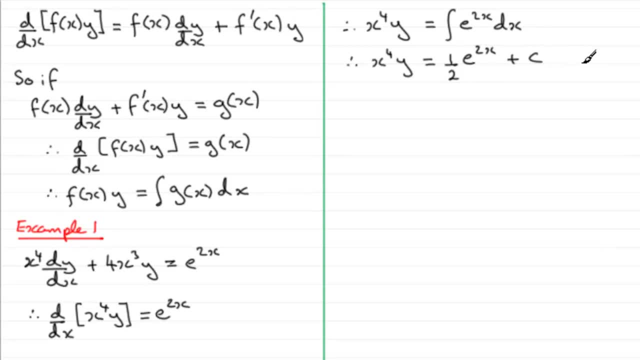 And then we mustn't forget the constant of integration. let's say plus c. Okay, well, that's how we go about solving that one. Now I've got another example here. you might like to try this one, Now that I've given you one to do. 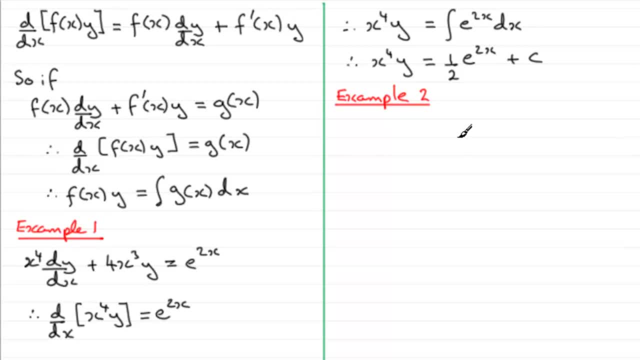 It's got a few other features in it though that might throw you- hopefully not, but it's worth giving it a try. This time we've got a trigonometric one. We've got cos x multiplied by dy, by dx minus y times the sine of x equals x squared. 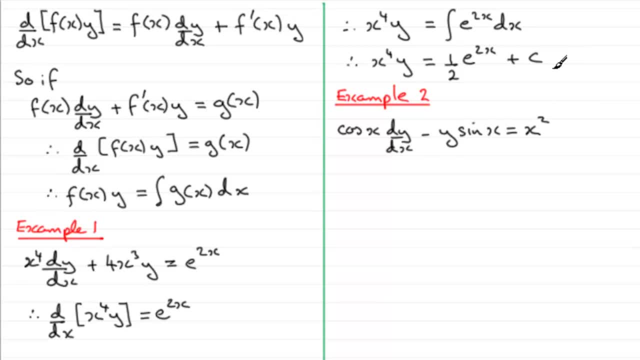 But when it gets to work- and we're working out this constant- I'm going to give you some boundary conditions. We're going to say, given that y equals 1 when x equals 0.. So you might like to give this a go, okay? 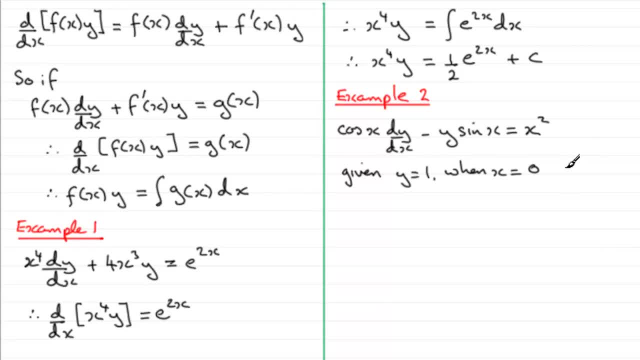 Just pause the video, come back when ready and you can check your work solution with mine. Okay, welcome back if you had a go at this. Okay, welcome back if you had a go at this. Let's see how you got on. 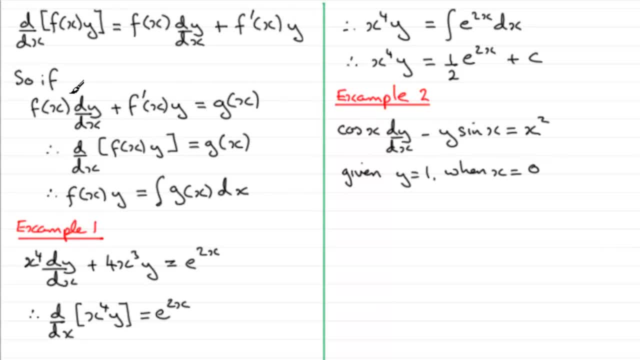 Well, first of all, this has got this format up here, Because if this is f of x cos x, then if I differentiate cos x I get minus sine x and you can see we've got minus sine x and then that's multiplied by the y. 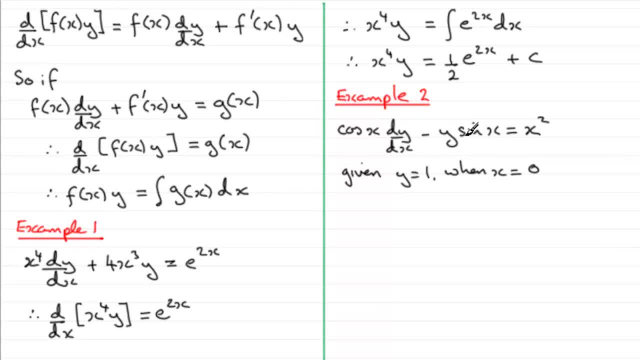 So we've got this term here, So that would mean that I can write: the left-hand side is the differential of a product. So, in other words, if we were to differentiate with respect to x, y, cos x, okay, I've written the y in front of the cos x this time. 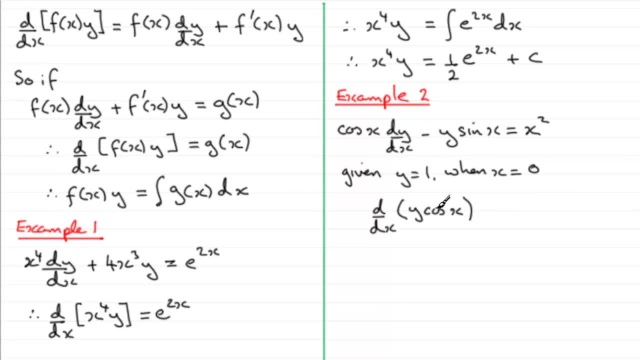 on purpose. it just looks better that way. But nonetheless, if you differentiate this by the product rule, you'll get the left-hand side here And this will equal x squared. So if I integrate both sides with respect to x, we've got that. therefore, y cos x must be equal. 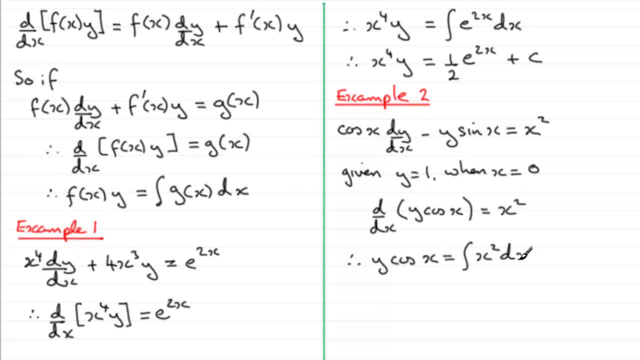 to the integral of x squared with respect to x. Now if I integrate x squared with respect to x, we've got y equals cos, x then equals a third x cubed, And then plus that constant of integration plus c. Now we know that we're told that when y equals one, 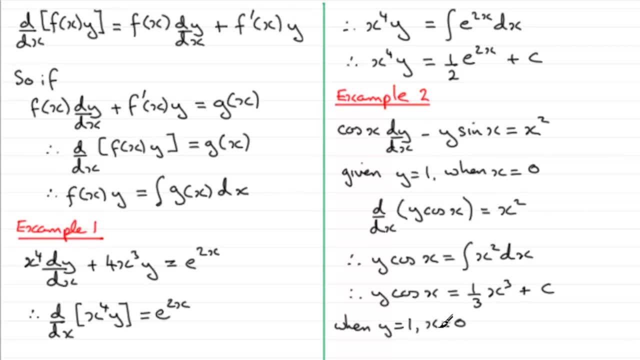 x equals zero, And if we substitute these values in to our equation up here, we're going to have one here multiplied by the cosine of zero. Cosine of zero is one, So you've got one times one, which is one equals. 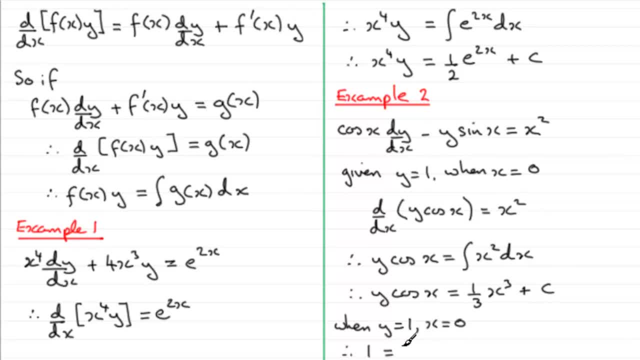 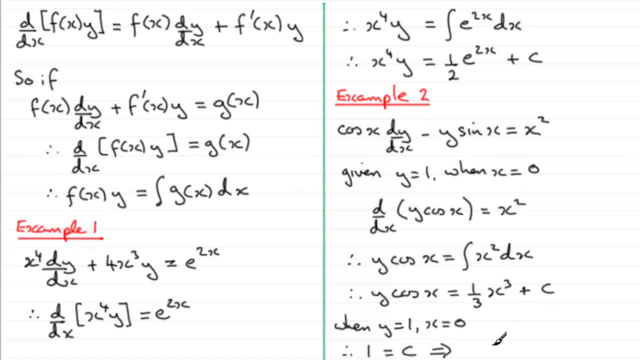 equation rather than the general solution. remember, general solution is when you have plus c in. it is going to be now: y cos x equals one third of x cubed, and then plus the value of c, which in this example is one. Okay, 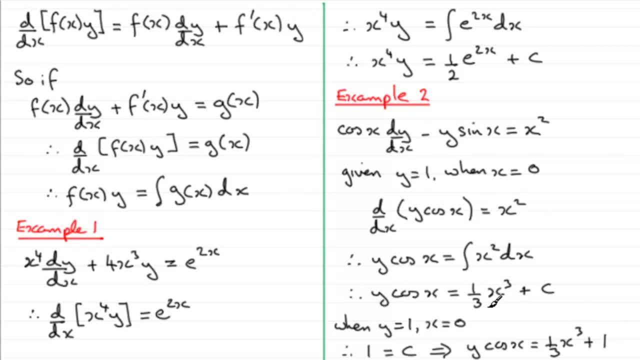 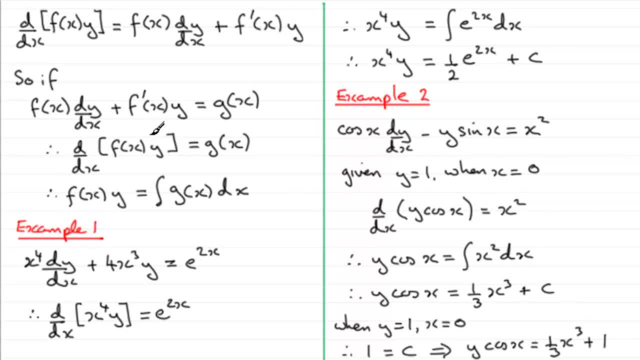 So I hope that's given you some idea then on these types of first equations. So I hope that's given you some idea then on these types of first equations. They're called exact equations. okay, when they have this particular format You can't separate the variables in them. 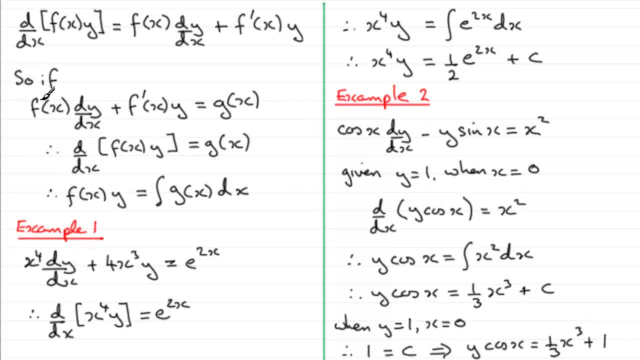 so you have to look for the possibility of this style for this to work. Okay, well, that brings us now, anyway, to the end of this particular video, so hopefully it's been of use to you. Don't forget: plenty more videos on my website. 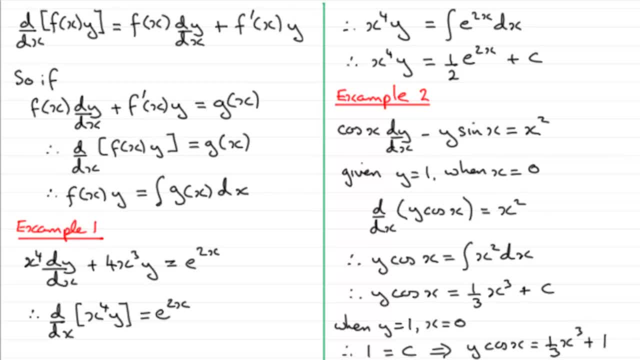 examsolutionsnet. Thank you.